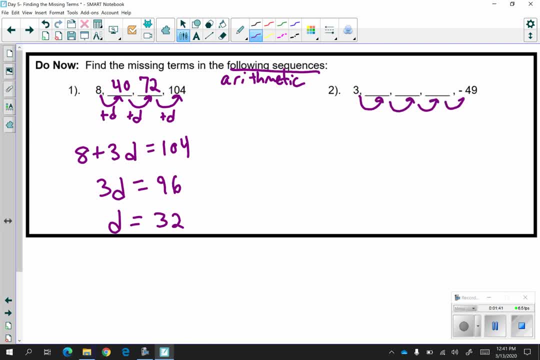 if you draw it out, you can see that you are adding a common difference four times because you're skipping four terms ahead, So 3.. Plus my four skips has to give me negative 49.. As you solve for D, you get that 4D has to be equal to negative 52.. 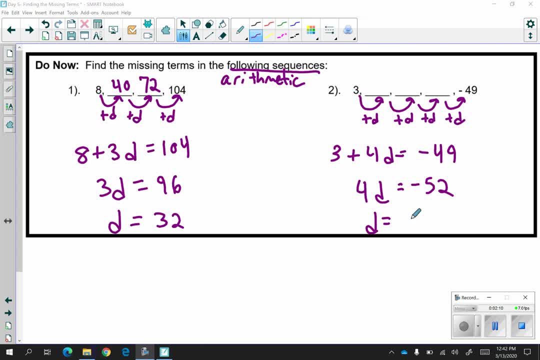 So that D has to be negative 13.. 3 minus 13, or 3 plus negative 13, would be negative 10.. Negative 10 minus 13 is negative 23,. minus another 13 is negative 36.. And that brings you again, when you do your final subtraction, to negative 49.. 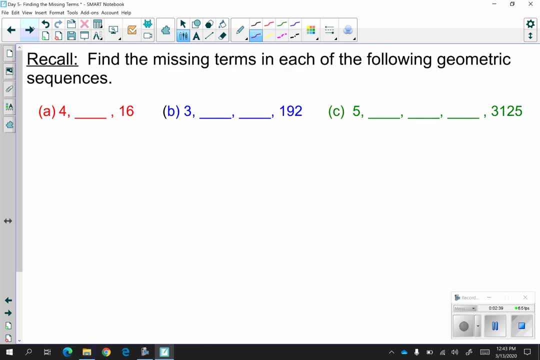 All checks out. Now let's look at geometric sequences. So, because they're geometric right, you don't have a common difference. Instead, you have a common ratio, an R. So you can see that you have a common ratio, an R. 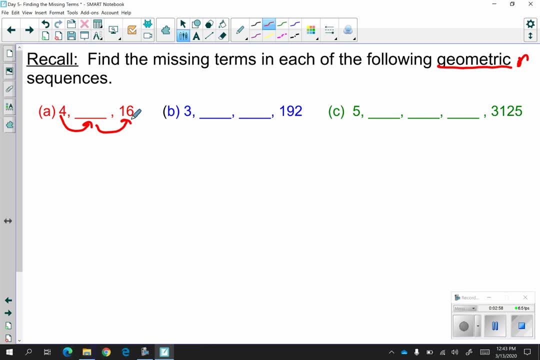 And now to get from one term to the next, not only are you going ahead by the common ratio, but in this case you are multiplying by the common ratio. So we're going to have 4 times R. times another R brings you to 16.. 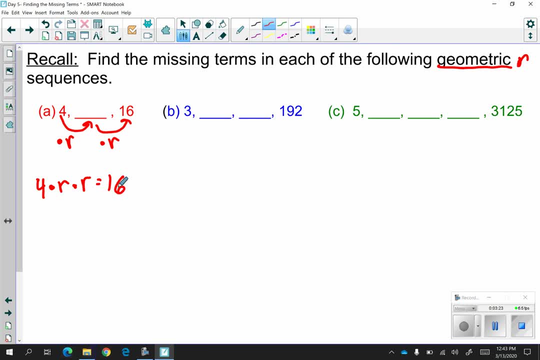 Now please don't write 4 as a common ratio. You don't have to. Times 2R brings you to 16, because R times R is R squared. So now we have 4. R squared is equal to 16.. 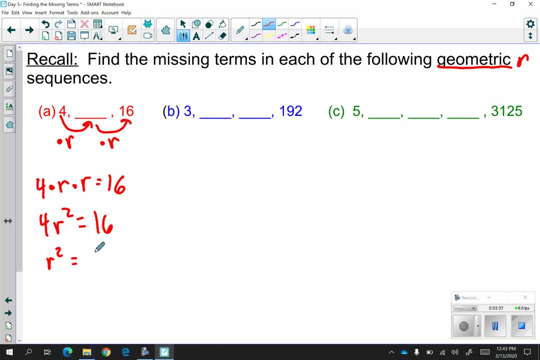 In other words, R squared has to be 4.. Keep in mind, when you take the square root, you need a plus or minus right. So we have: R is equal to plus or minus 2.. Let's start with the plus right. 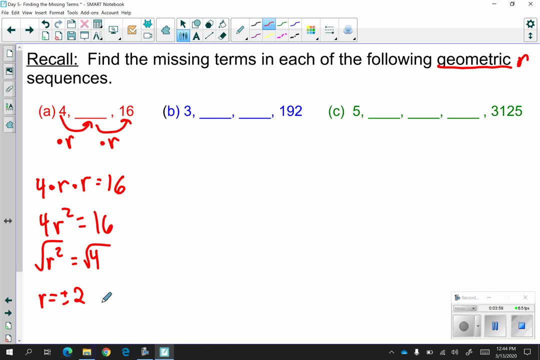 Your first case is times positive, 2.. So 4 times 2 is 8.. 8 times 2 is 16.. Now let's say you went with the negative 2.. 4 times negative, 2 is negative, 8.. 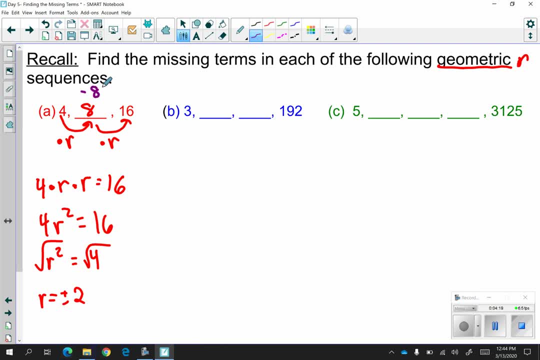 And negative. 8 times negative, 2 would give you positive 16.. So the thing is, when you have a geometric sequence, you can actually potentially have two different answers. right, Because you can go between positive and negative, positive and negative, positive and negative. 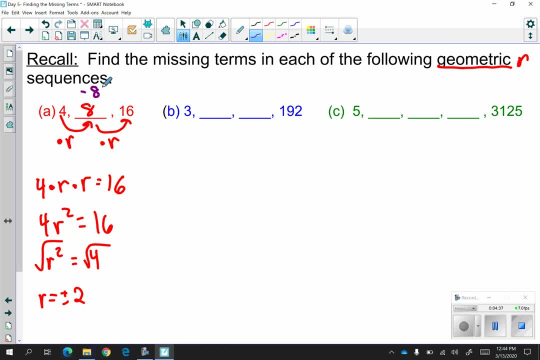 if your common ratio is negative, or you can just keep the same sign each time. if you have a positive common ratio, Let's try the next one. We're skipping one, two, three times. So we have three times the three R's that we're skipping. 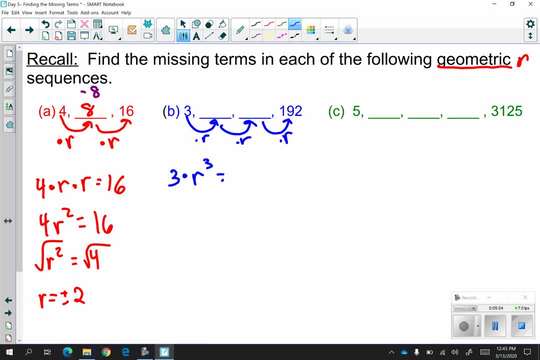 So R times R times R is R cubed equals 192.. As you go to solve, you have that R cubed is equal to 64.. Okay, And to get rid of R cubed you have to take the cubed root of both sides. 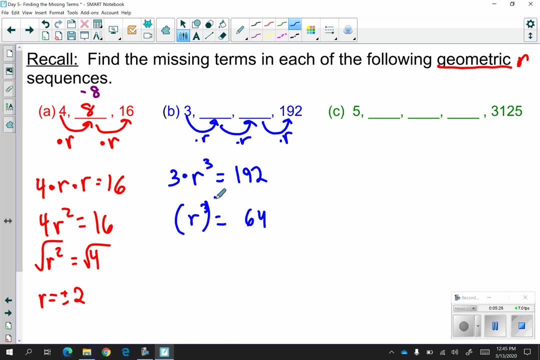 If you don't want to do the cubed root, you could also raise it to the reciprocal power. The choice is yours. Either way, you want to do it same answer. The point is that R will end up being 4.. You're not going to put a plus or minus this time. 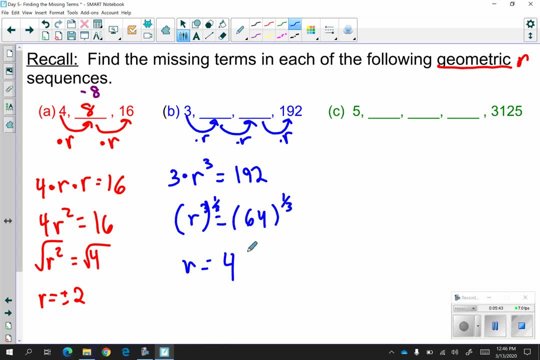 because you only include the plus or minus if you're taking an even root, if you're taking an even root, If you're taking an odd root, such as the cubed root, no plus or minus, So you only have one answer. 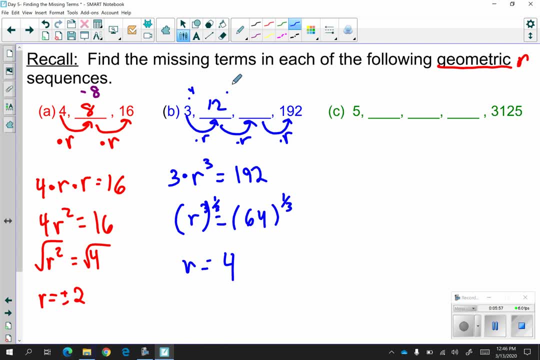 Three times four will give you 12.. Times another four will give you 48.. Times another four will bring you to 192.. That way you did everything properly And let's try the last one. Okay, Let's see, Let's see. 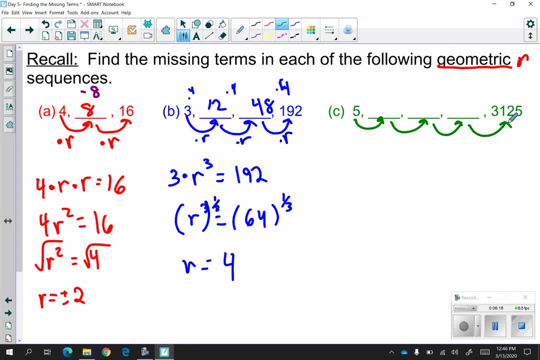 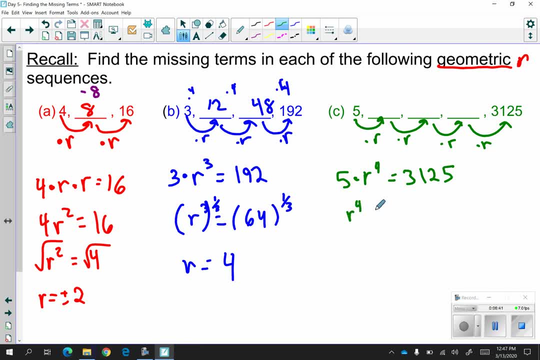 If you divide by 5 on both sides, you get that R to the fourth power is equal to 625.. Yeah, 25.. And then when you take the fourth root, or if you want to raise both sides to the 1 over 4,, 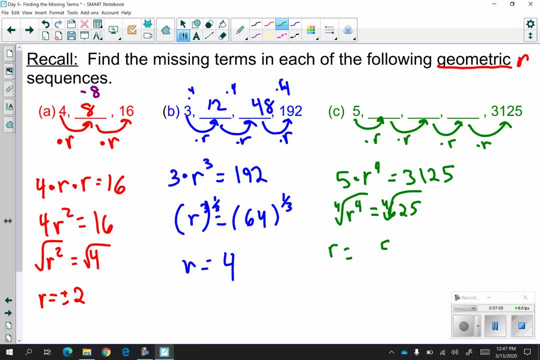 you should be getting in your calculator 5.. Now, if you want to take the root in your calculator, hit math and it'll bring you to an option where it has x root, And if you choose the x root option, you'll be able to plug in what root number you want to take for x. So keep in mind you took an. 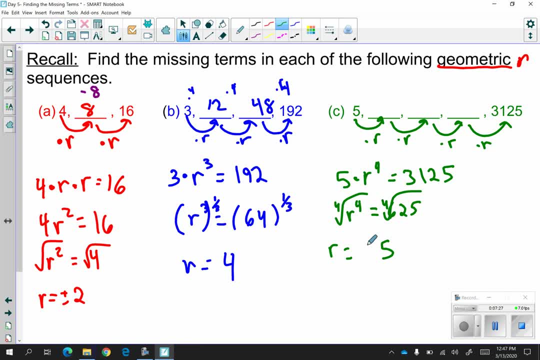 even number of root right. Our index was 4.. Because it's even. you need a plus or minus. Let's work with the pluses first right. If you had, r is equal to positive 5, let's look at what our answers would be. We would have 5 times 5, which is 25,. 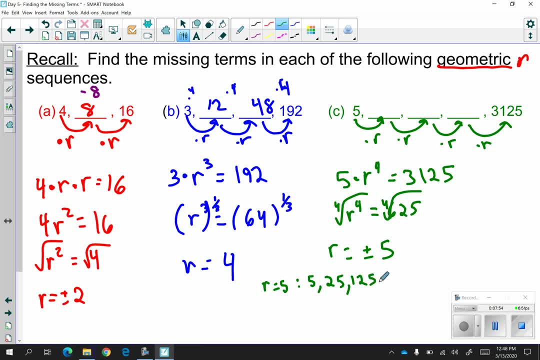 times another 5, which brings you to 125,, times another 5,, 625, and times another 5 brings you to your final term of 3125.. If you had, r is equal to negative 5, and we're starting with 5,. 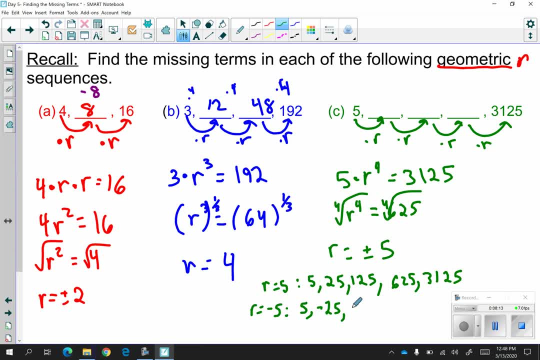 times another 5, which brings you to your final term of 3125.. negative 5 is negative 25, times. another negative is positive 125, times another negative is negative: 625, and then we're back to positive 3125. 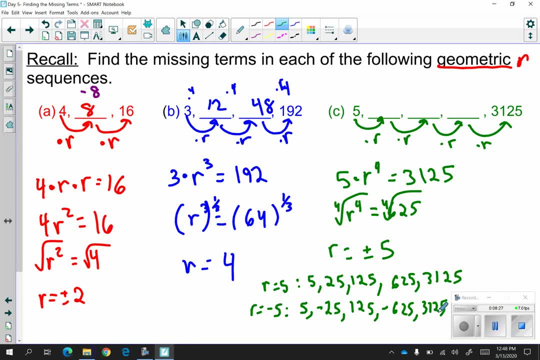 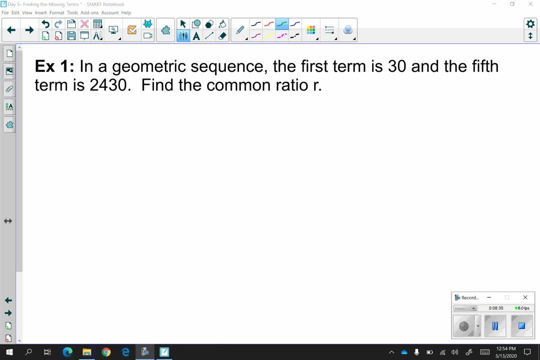 So just keep in mind that negative answers will cause your sequence to oscillate back and forth between negative and positive. So why don't you try this example on your own and then check back to see if you got the correct answer? Hopefully we have the right setup, right. 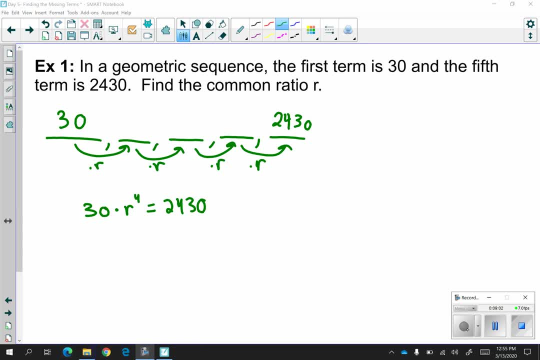 You're starting with 30, you are making 4 skips, so you have r to the 4th and then you're being equal to 2430.. If you continue to solve for r, remember, if you don't want to do the 4th root, you can. 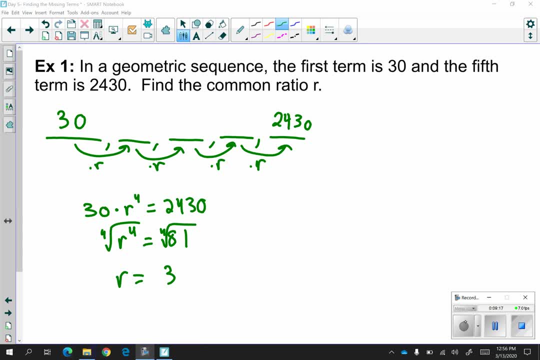 raise it to the 1 over 4 power, but then, because you're taking an even root or the denominator of your exponent is even, you need to include a plus or minus, And then you're done, because the problem is not asking for what are the missing terms? 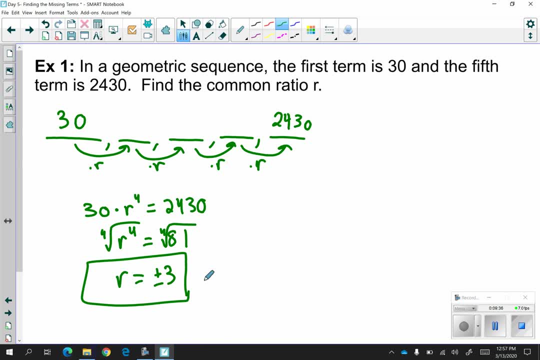 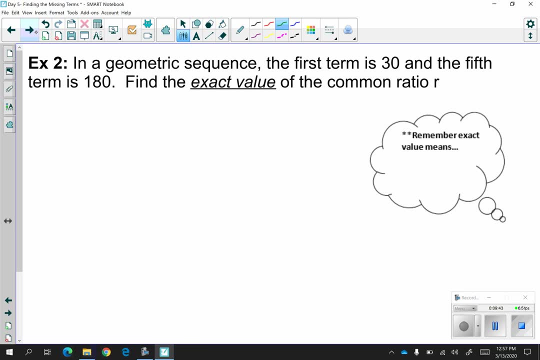 they're asking for what's the common ratio r, and you figured it out, So for this problem, try it again on your own, but keep in mind it's asking for the exact value, And remember that exact value means you don't want decimals, so keep that in mind. 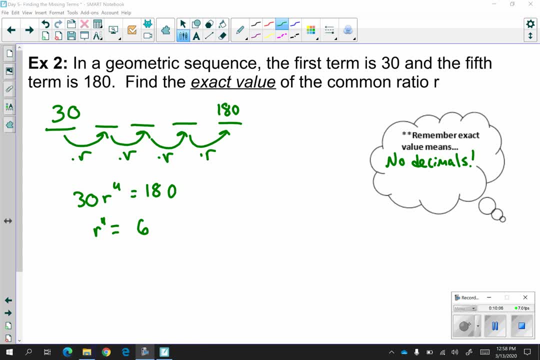 So as you solve for this, you should be getting that r to the 4th, And then when you go and take the 4th root, you have that r is equal to something that becomes a decimal on your calculator, right? because you can't take the 4th root of 6.. 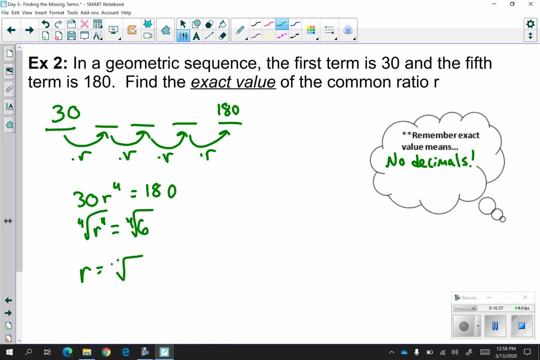 So you're going to leave it as the 4th root of 6.. Of course, with a plus or minus, because you took an even root. Your other answer could be that: So you're going to leave it as the 4th root of 6.. Of course, with a plus or minus, because you took an even root. Your other answer could be that: 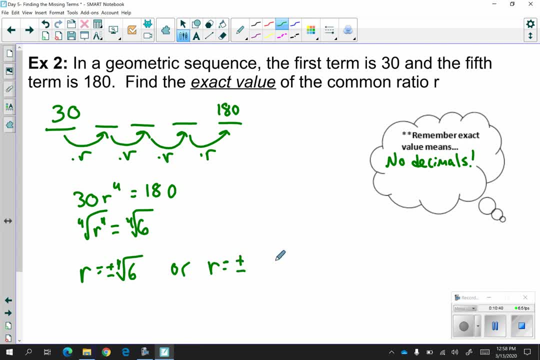 You have plus or minus 6 to the 1 over 4th power. Just make sure you write it and make sure it's tiny as an exponent. So keep in mind that exact value means no decimals and you want to leave the answer in radical form. 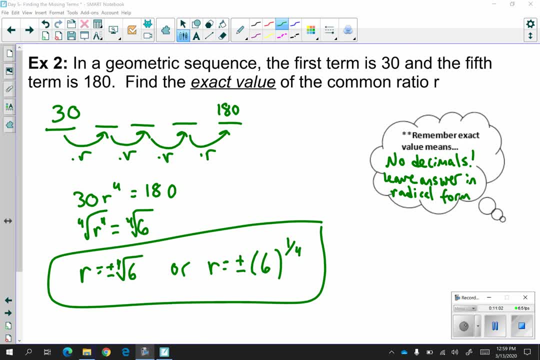 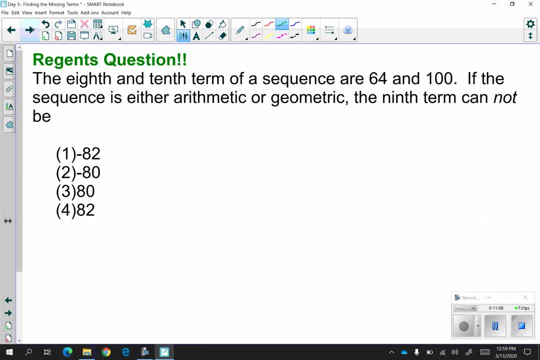 I should also say that you can leave your answer in rational form if you choose to do it this way. Now let's look at an actual region's question. So in this question, try to figure out why this one is different than the previous. 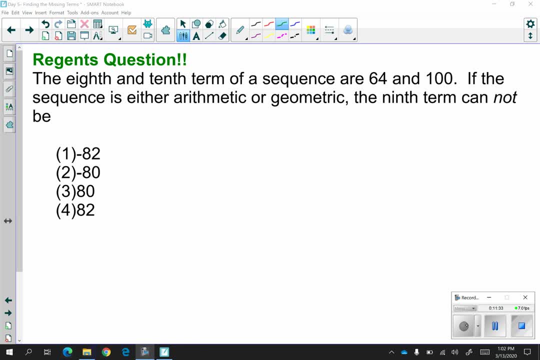 They're starting off by telling you that you have the 8th and 10th term. So the 8th term is 64.. Don't know what the 9th term is, but you know that the 10th term is 100.. 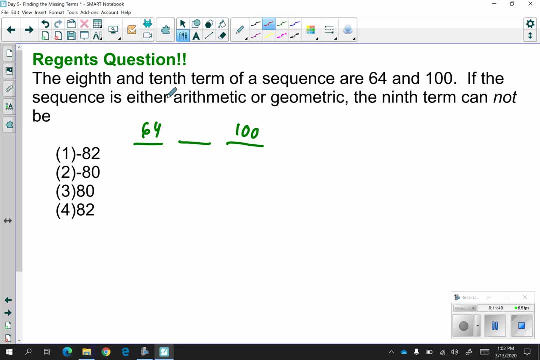 They're saying in this one- which is why it's different- is that it's either arithmetic or geometric. They're not telling you what it is, But they're asking for which. one will not work as your 9th term, So you kind of have to do it both arithmetically and geometrically to figure it out. 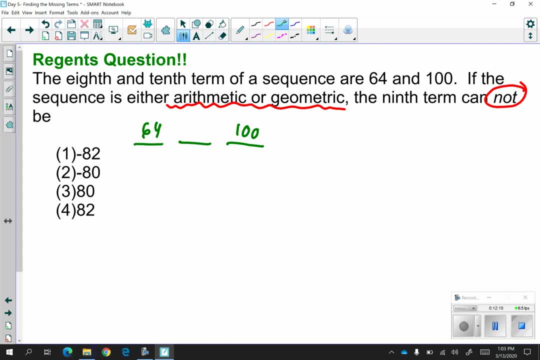 So Pause the video, Figure out what it would be if it was arithmetic, and then figure out what it would be if it were to be geometric. You gotta do the problem twice. So keep in mind when you get your common difference and your common ratio. 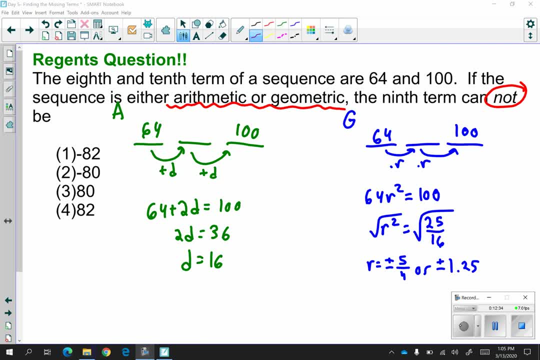 you're not done with the problem because that's only telling you what the patterns are. You actually have to go back and figure out what the 9th term is. So we have that in the green one, your arithmetic sequence If the common difference is 16,. 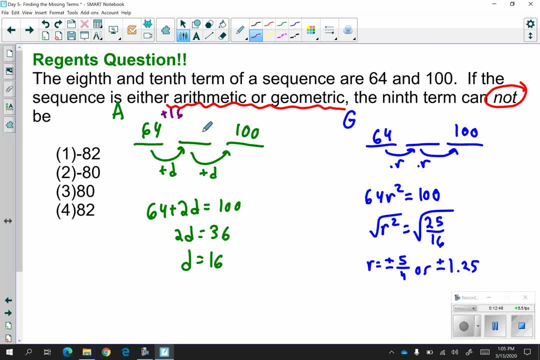 then 64 plus 16 will bring you to 80, 80. Oh sorry, it's not going to be 16,, it's going to be 18.. That's why things weren't working out, So your common difference would be 18.. 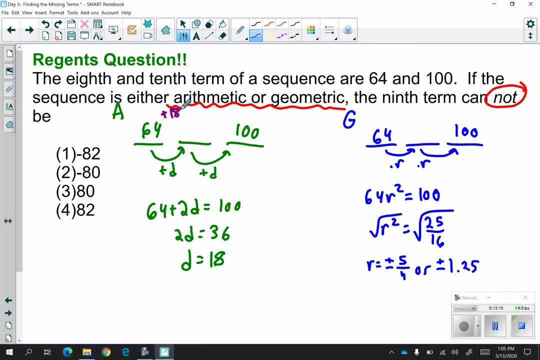 You have that you're adding 18 each time and 64 plus 18 is going to bring you to 82. And then 82 plus another 18 would bring you to 100. So we know that 82 works. You can cross it off the list. 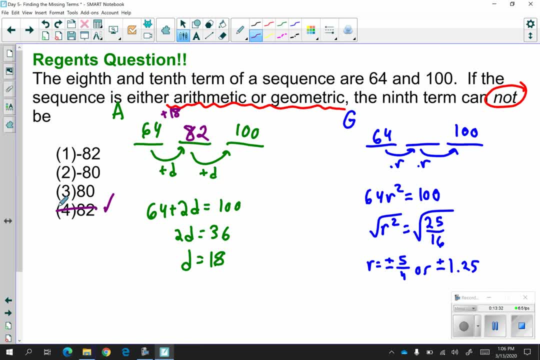 On the other side for geometric you got plus or minus 1.25.. So 64 times 1.25 will bring you to 80. And 64 times negative 1.25 will bring you to negative 80. So you get those two answers: positive 80 and negative 80, both work. 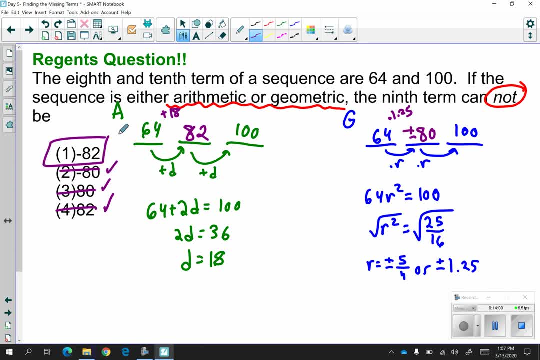 which means negative. 82 is the one left out. Now. did you have to do all this work? No, Because you should know that here any time they give you these types of problems. there's really going to be two that are geometric. 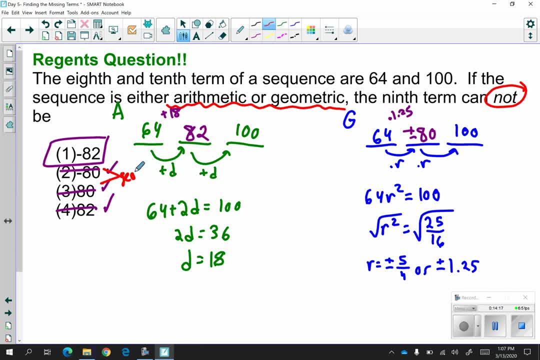 because geometric answers can always be positive or negative, And there's going to be two that are going to be, if you were to do it arithmetically. But the thing is, arithmetic sequence can only have one common difference. right, You can't add 18 and subtract. 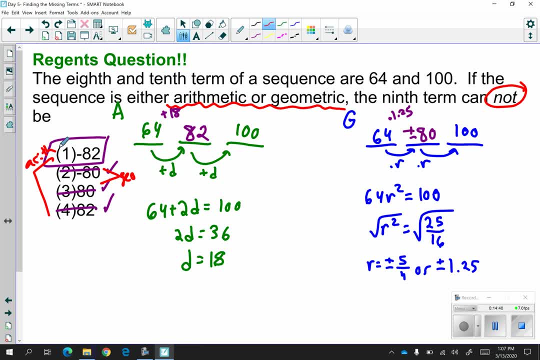 You can't subtract 18 and have it still work. So, in reality, none of the geometric had to be done, because it's always going to have those two answers for these types of problems. All you really had to do was the arithmetic work. 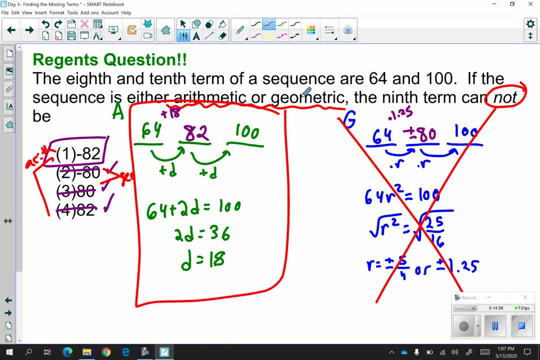 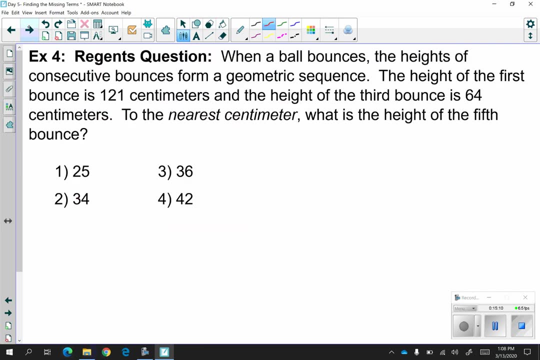 Because if you did this and you realized that your common difference was positive 82,, that should have gave you an indication that negative 82 wouldn't have worked. So let's try one more problem, because this was a region's question and it tripped up a lot of people. 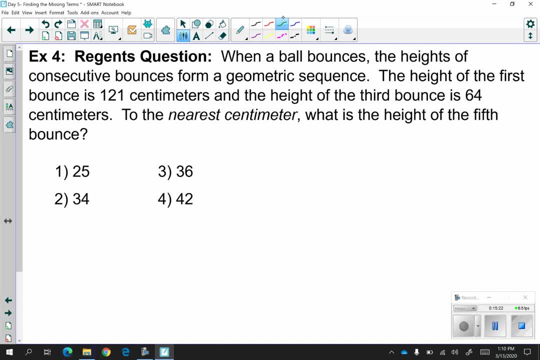 We're talking about when a ball bounces. the heights of consecutive bounces form a geometric sequence, So we know that we have a common ratio. We have the height of the first bounce, which is 121.. And the height of the third bounce. 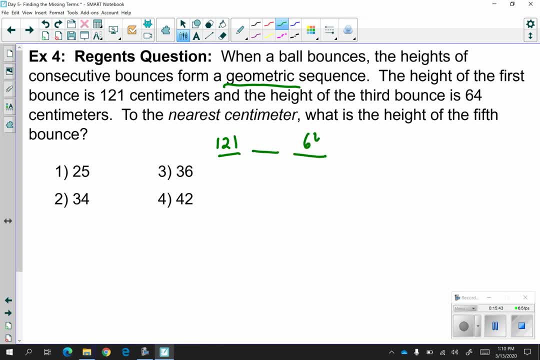 So we're skipping the second. We know that the third is 64. We want to figure out to the nearest centimeter what's the height of the fifth bounce. So they're trying to figure out what is this guy? Now, before you can figure out the fifth bounce, 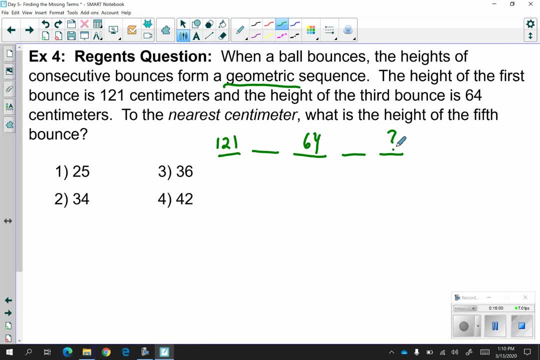 you have to figure out what your common ratio is, And for that you need the first through the third bounces. So we have that we're skipping twice with the values that we know, And you can set up the equation 121 times two skips got me to my third bounce. 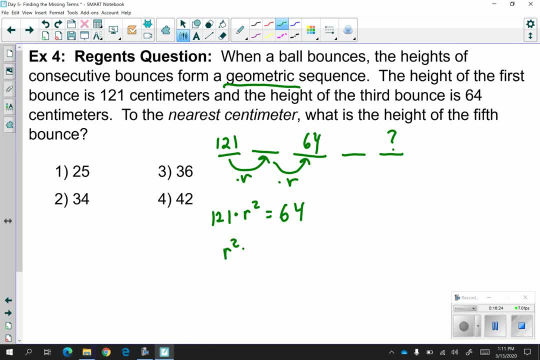 So you're going to have that r squared is equal to 64 over 121.. Or when you take the square root of that, you're going to get that r is equal to plus or minus 8 over 11.. Now, if you think about this realistically, 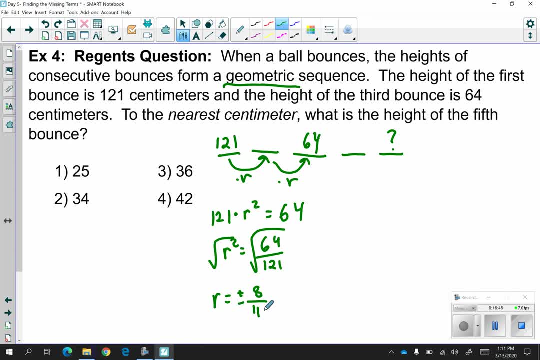 we're talking about the height of a bounce And you can't have negative height. So, even though you should be getting a plus or minus from the even root, don't include the minus, because it doesn't make sense in terms of this problem. 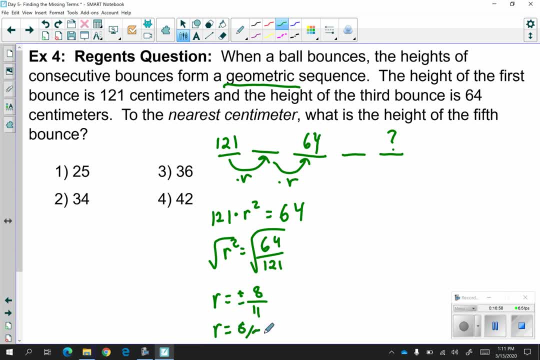 So we're really only dealing with 8 over 11.. Now that you know your common difference is 8 over 11, you're going to take 64, and in your calculator, you're going to multiply it by 8 over 11.. 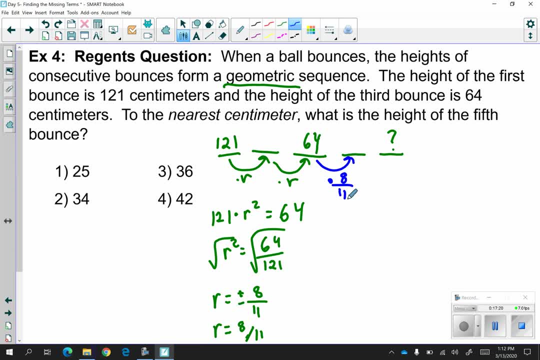 And please make sure that when you're doing this, 8 over 11 is a fraction. Please do it using alpha y equals. make it a fraction, exactly like what you would do if you were to write it out on paper. You should be getting 512 over 11.. 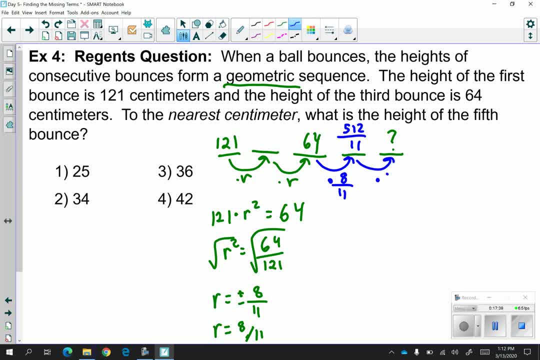 And then you're going to multiply by another 8 over 11.. When you do that, you should get 4,096 over 121.. Now, obviously, that answer is not there. So if you were to take 4,096 over 121 and convert it into a decimal, 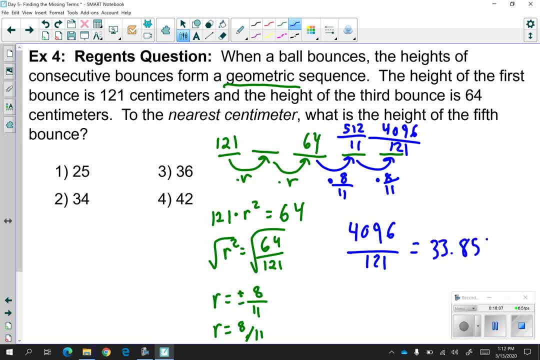 you should be getting 33,, 8,, 5,, 1,, 2, and so on. It continues, And obviously 33.8 rounds to 34.. So why don't you work through the packet? Work on the practice section.